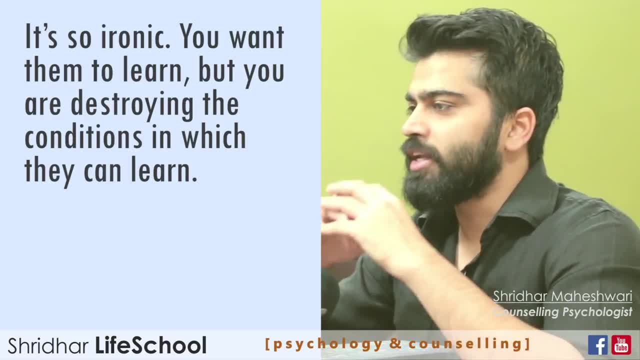 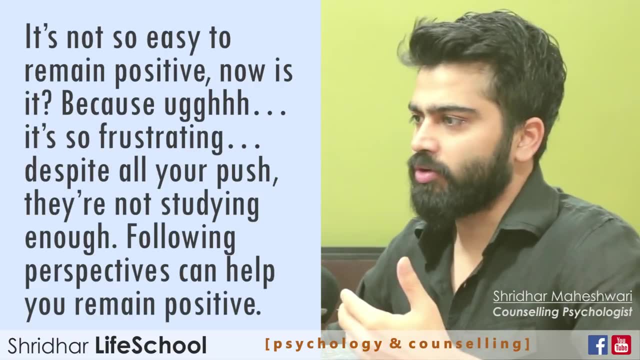 emotions and you increase stress. How do you expect them to learn? well, It's so ironic – you want your child to learn, but you're destroying the conditions in which they can learn. It's not so easy to remain positive now – is it Because it's so frustrating? 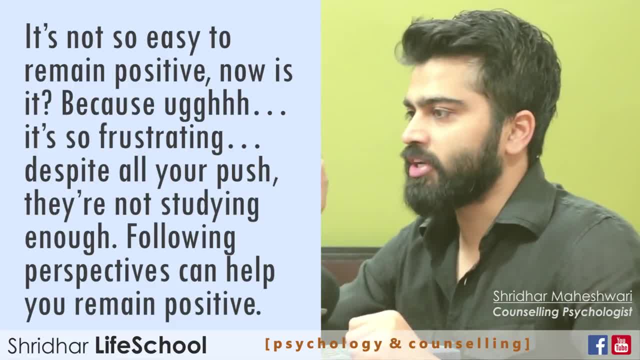 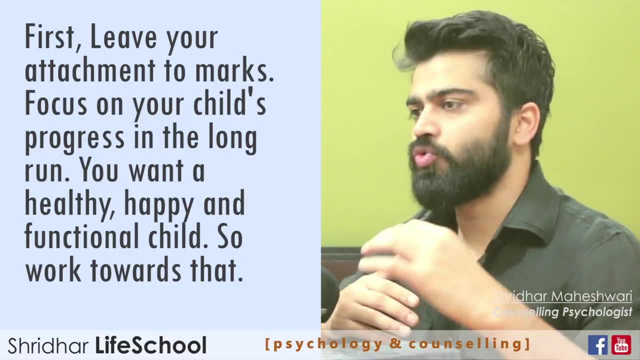 despite all your push, they're not studying enough. Following perspectives can help you be positive. Leave your attachment to marks. Focus on your child's progress in the long run. You want a healthy and happy and functional child – so work towards that. It's really hard to leave. 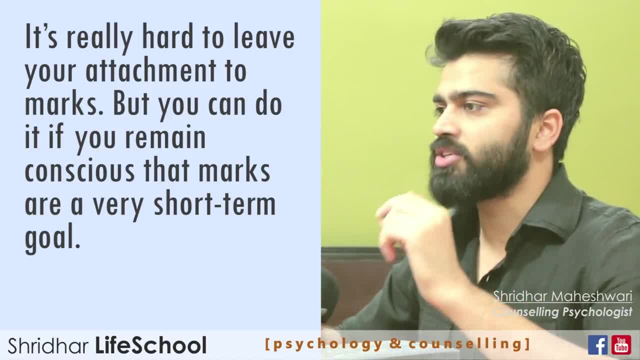 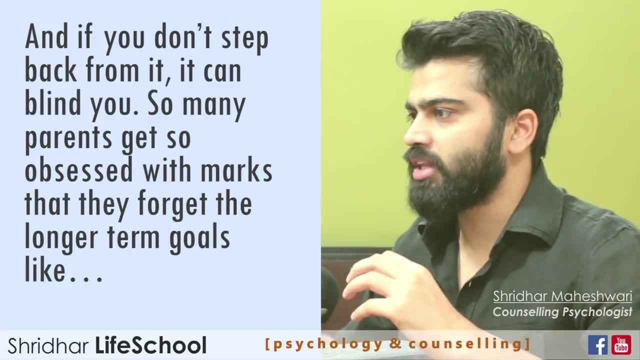 your attachment to marks. but you can do it if you remain conscious that marks are a very short-term goal and if you don't step back from it, it can blind you. So many parents get so obsessed with marks that they forget the long-term goals, like the child's actual learning, their sleep diet. 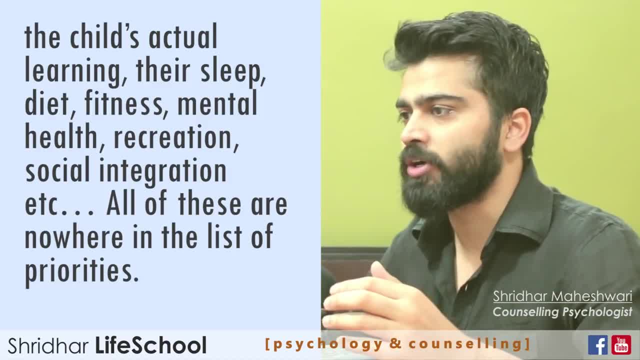 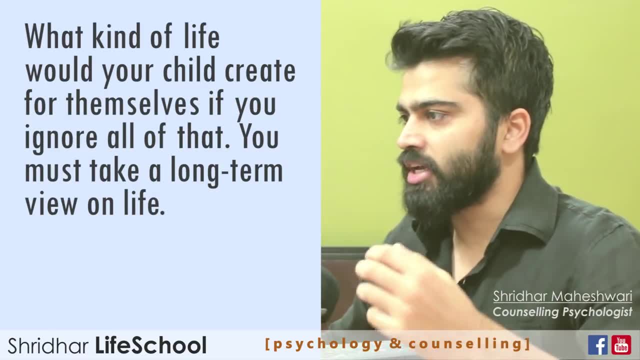 fitness, mental health, recreation, social integration, etc. All of these are nowhere in the list of priorities. What kind of life would your child create for themselves if you ignore all of that? You must take a long-term view on life. So if you focus on the bigger picture and let go of 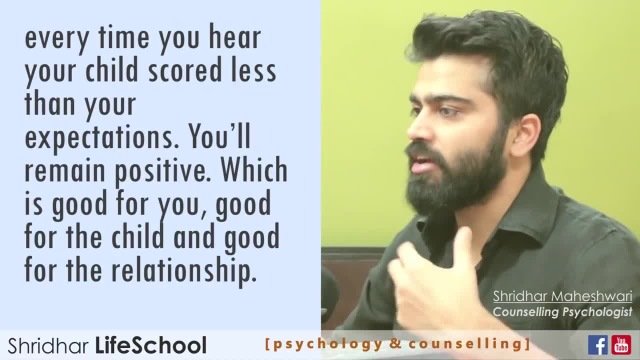 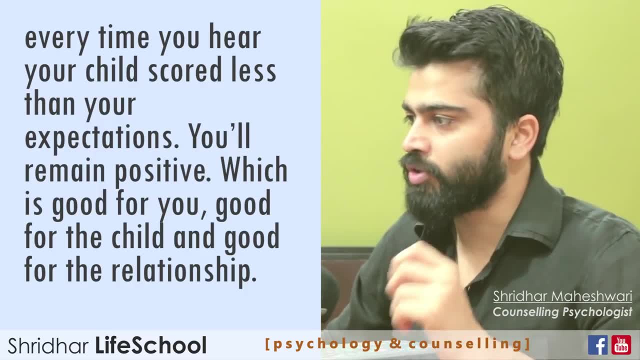 the attachment to marks. you won't suddenly become disappointed or angry every time you hear your child scored less than your expectations. You'll remain positive, which is good for you, good for the child and good for the relationship. Second, many parents fear that my child simply isn't. 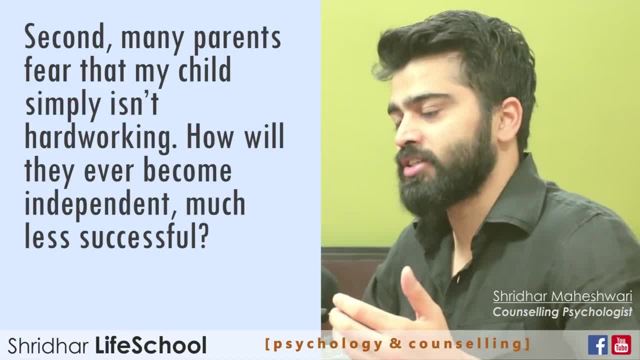 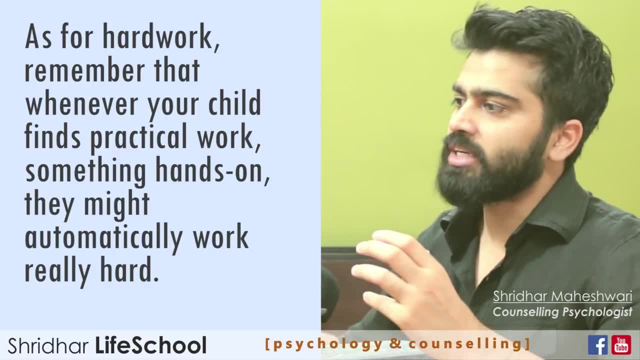 hard-working, How will they ever become independent, much less successful. As for hard work, remember that whenever your child finds practical work, something hands-on, they might automatically work really hard. School books, inherently, are not good at generating motivation to work hard. 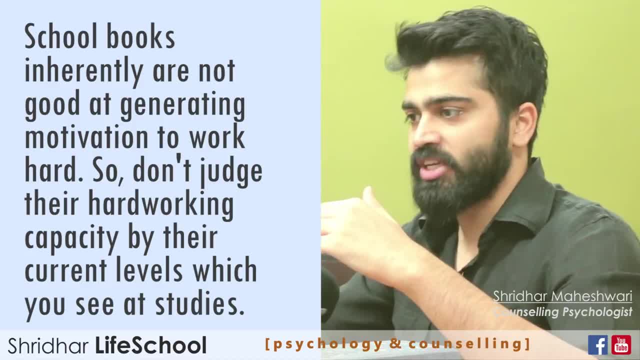 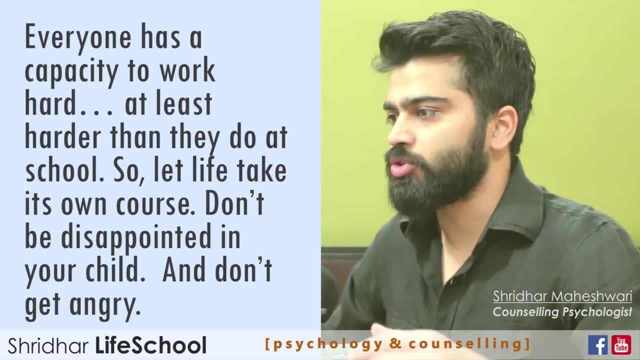 So don't judge their hard-working capacity by their current levels, which you see at studies. Everyone has a capacity to work hard, at least harder than they do at school. So let life take its own course. Don't be disappointed in your child and don't get angry. Finally, just remember. 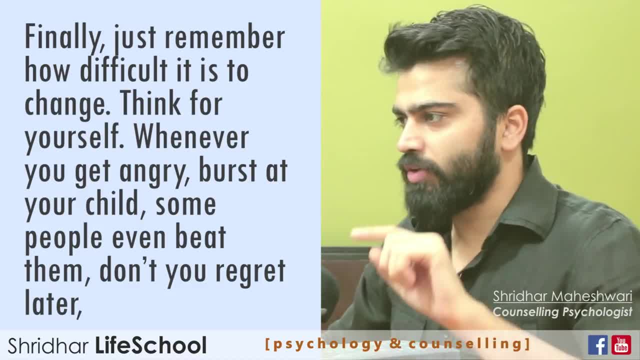 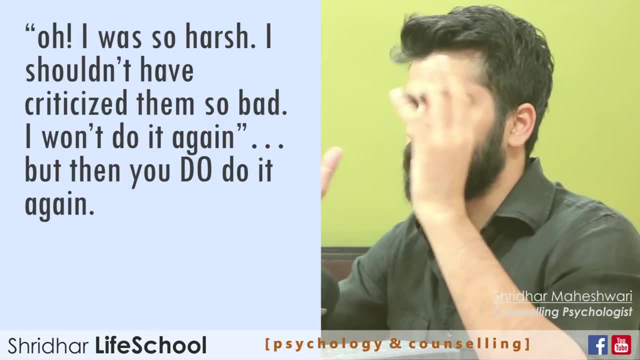 how difficult it is to change. Think for yourself whenever you get angry burst at your child. some people even beat them. Don't you regret later: oh, I was so harsh, I shouldn't have criticized them so bad, I won't do it again. But then you do do it again If you can't change your.